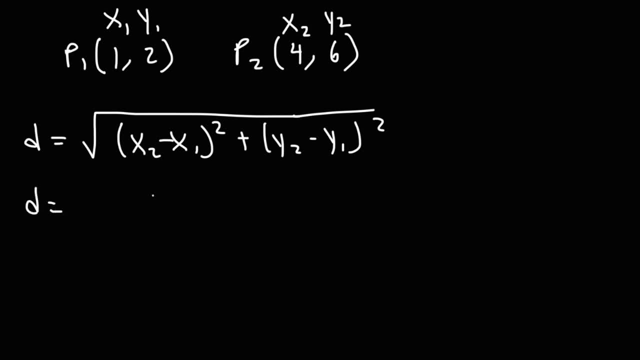 So what we need to do at this point is plug in the numbers into the formula. So x2 is 4, x1 is 1, y2 is 6, y1 is 2.. And now let's do the math. 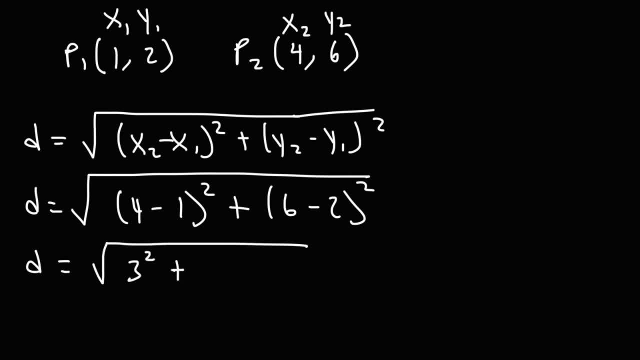 So 4 minus 1 is 3.. 6 minus 2 is 4.. 3 squared, that's 3 times 3,, which is 9.. 4 squared is 4 times 4,, which is 16.. 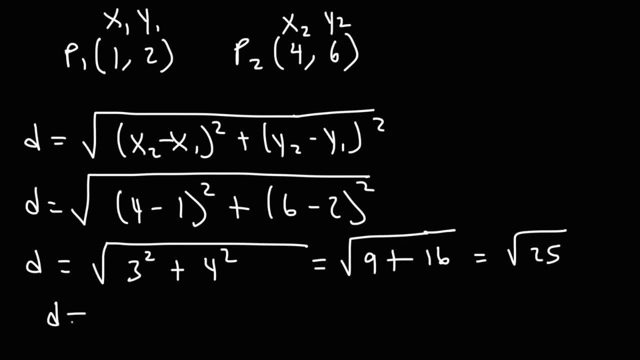 9 plus 16 is 25.. And the square root of 25 is 5.. So that is the distance between these two points. Now, another way in which you can get the answer is you can actually graph a picture to find the answer. 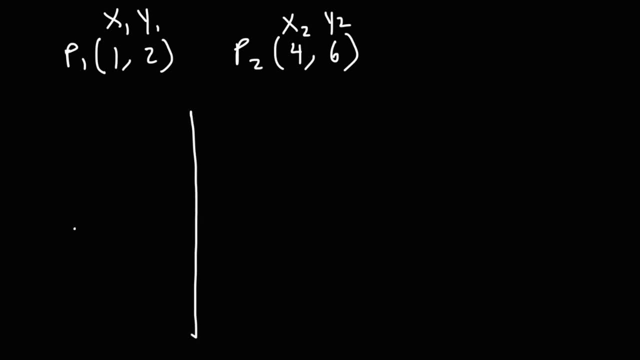 So let me show you That is not a straight line. Let's do that one more time. Now let's plot the points. So p1 is that 1, 2.. So the x value is 1, the y value is 2.. 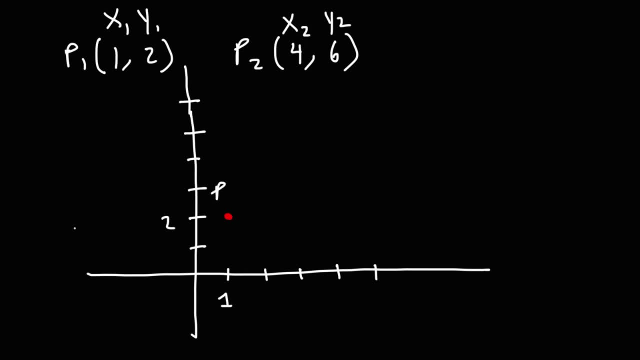 So that's our first point. Now the p2 is that an x value of 4 and a y value of 6.. So p2 is right here And we want to calculate the distance between those two points, And what we can do is we can form a right triangle. 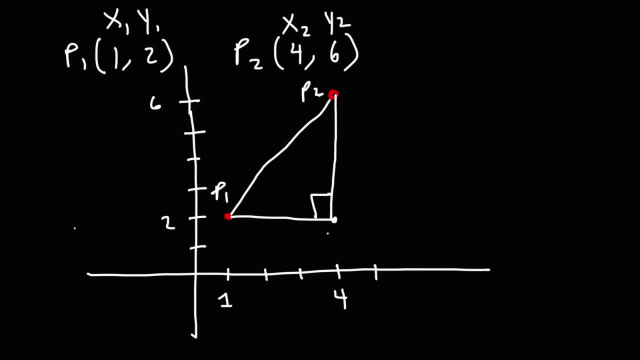 so, in order to go from p1, for each point here, p 10.. to this point, we need to travel 3 units to the right, And in order to go this direction- to get to P2, we need to travel from 2. 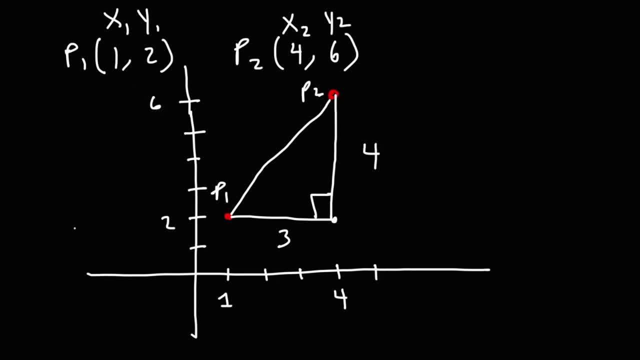 to 6, or 4 units up. So all we need to do is find the hypotenuse of the right triangle And we could use the Pythagorean theorem to get that answer. This is A, B and C. So in this example, A is 3,, B is 4, and we're 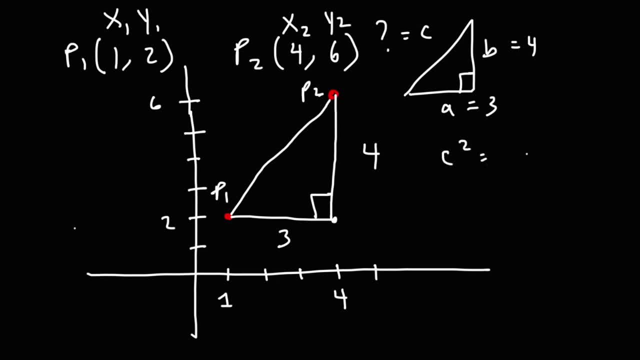 looking for C. So according to the Pythagorean theorem, C squared is equal to A squared plus B squared, So that's 3 squared plus 4 squared, And so we get 9 plus 16, which is 25.. And then taking the square root of both sides gives us the value of